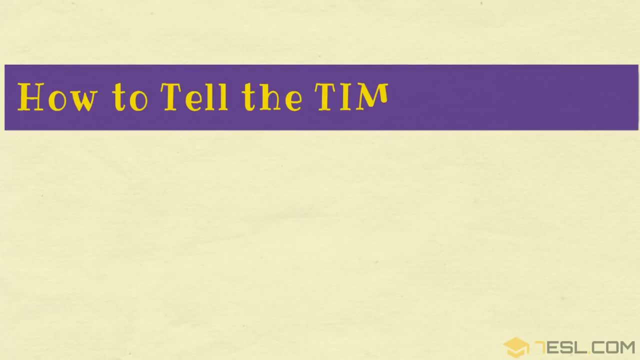 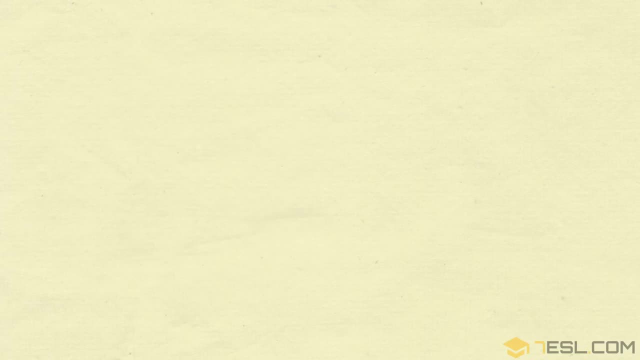 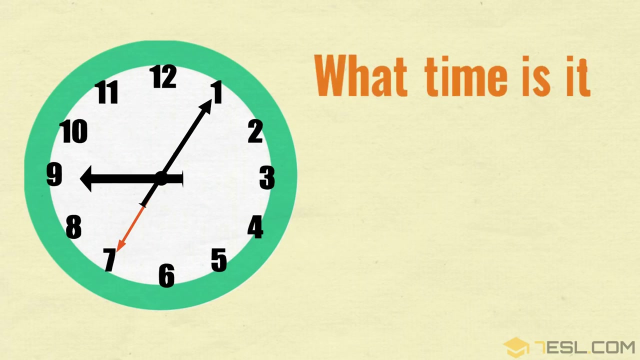 How to tell the time in English. What time is it? 9 o 5, or it's five past nine. 9, ten or it's ten past nine. 9, fifteen: it's quarter past nine. 9, twenty- it's twenty past nine. 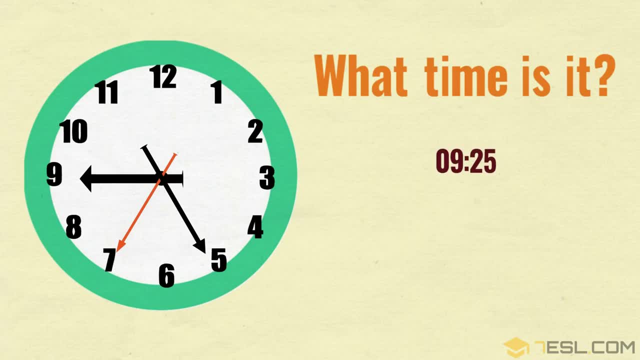 9, twenty-five. it's twenty-five past nine. 9 thirty. it's half past nine. 9 thirty-five. it's twenty-five to ten. 9 thirty-five. it's twenty-five to ten. 9 forty. it's twenty to ten. 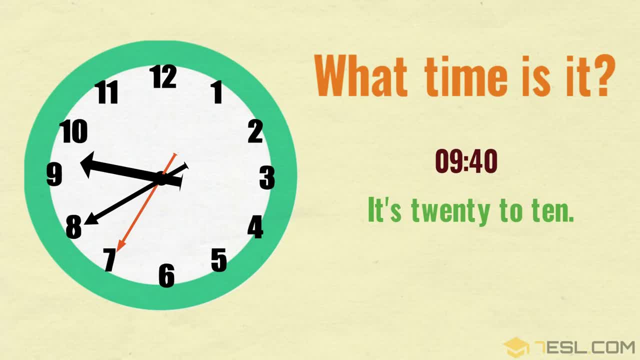 9, forty-five. it's quarter to ten: 9, fifty. it's ten to ten: 9, fifty-five. it's five to ten: 9, fifty-five. it's five to ten. 10 o'clock. it's ten o'clock. 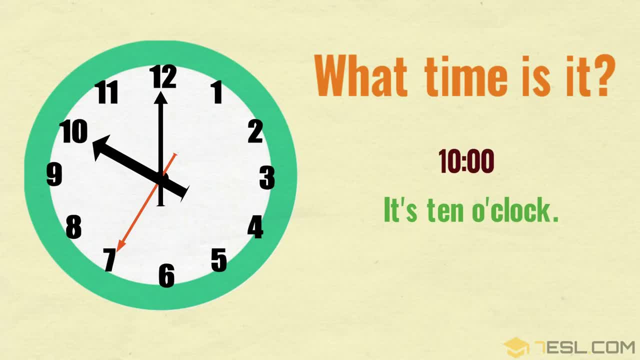 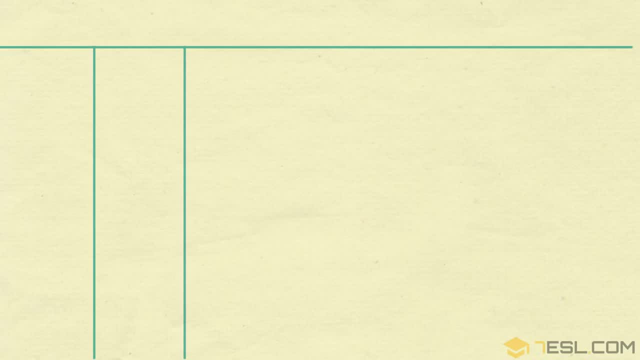 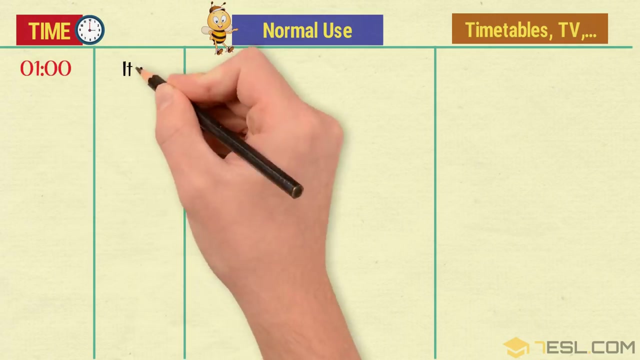 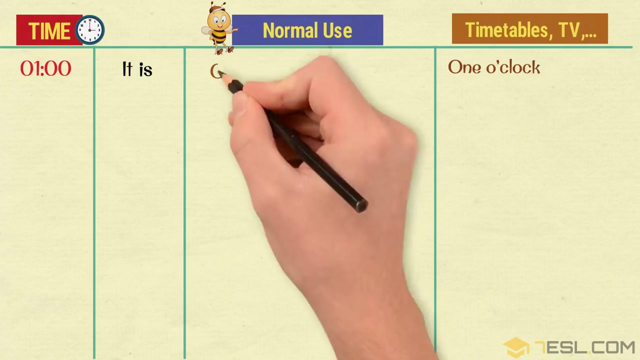 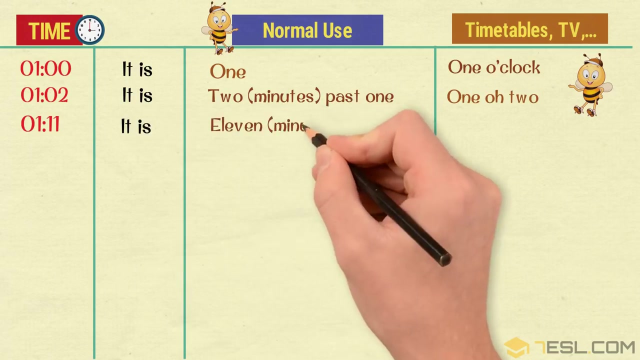 10 o'clock, it's ten o'clock, It is 1 o'clock, It is one o'clock. One. 1, 1 o'clock. 1 o'clock. 2 minutes past 1.. 1-0-2.. 11 minutes past 1.. 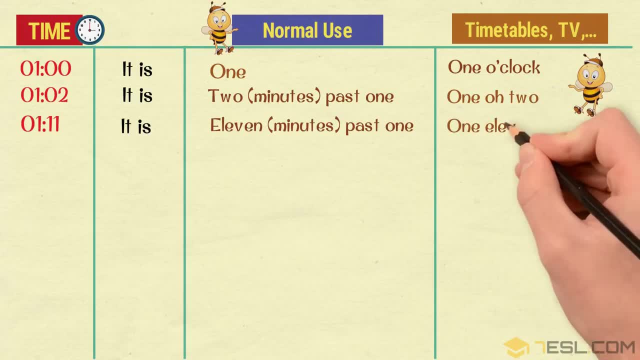 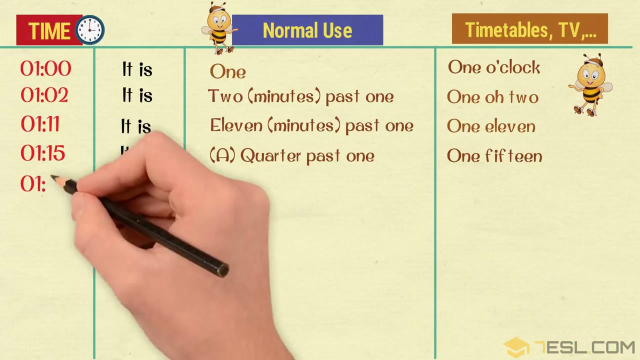 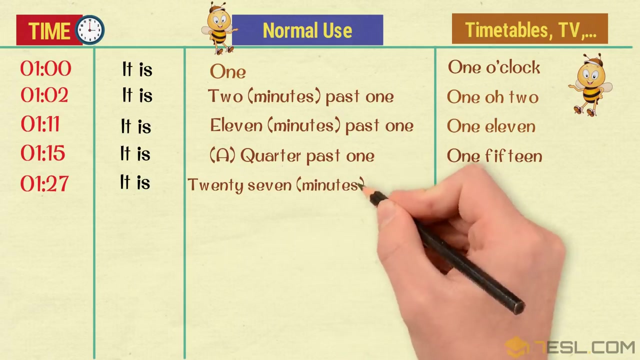 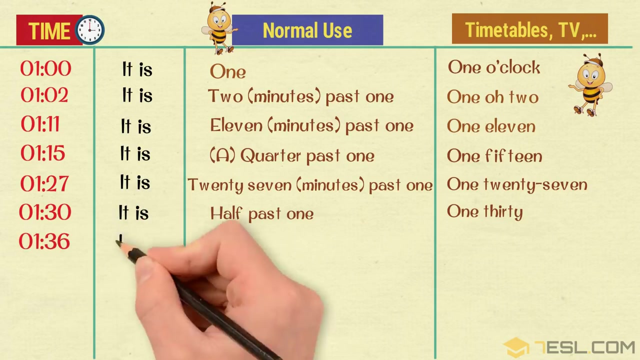 1-11.. A quarter past 1. 1-15.. 27 minutes past 1. 1-15.. 1-15.. 1-27.. Half past 1. 1-30.. 24 minutes to 2.. 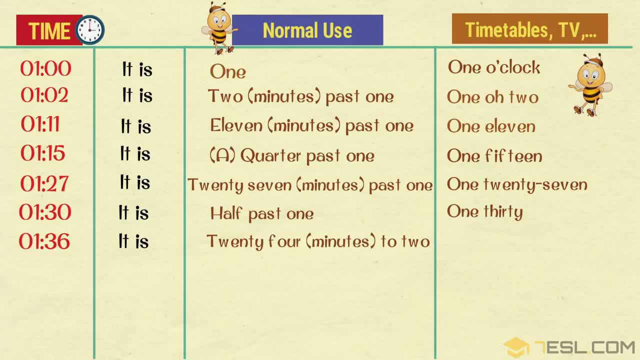 1-2.. 1-2. 1-2. 1-3.. 1-3.. 1-3.. 2 minutes past: 1. 1-2. 1-3.. 1-6.. 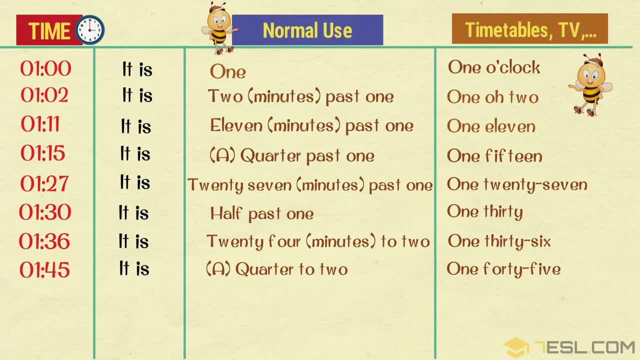 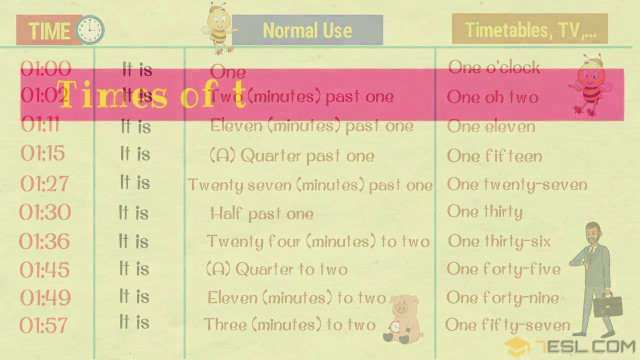 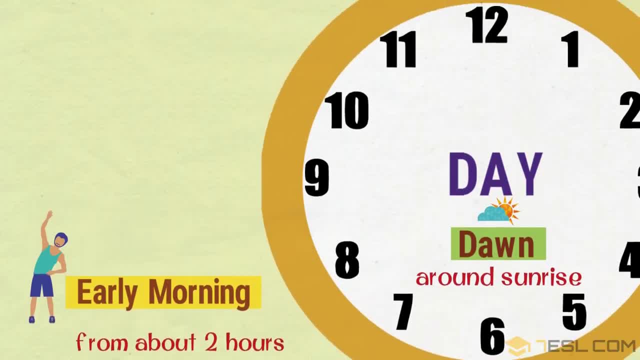 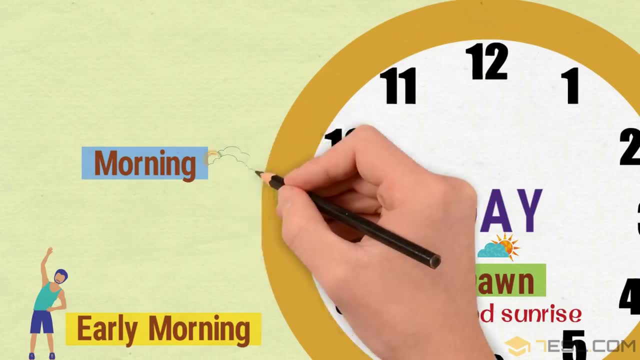 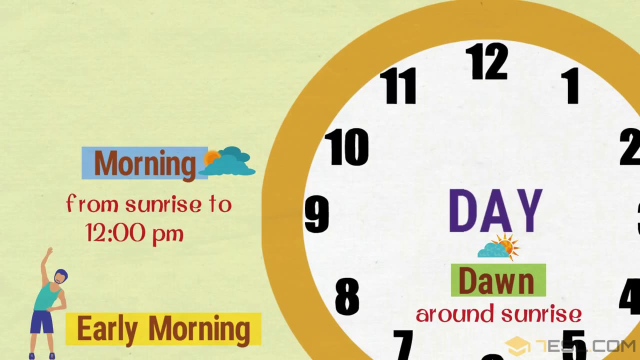 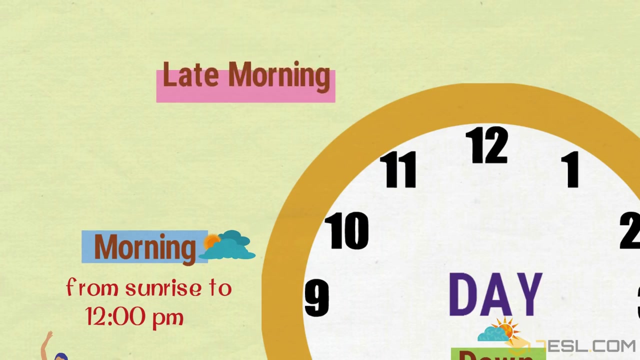 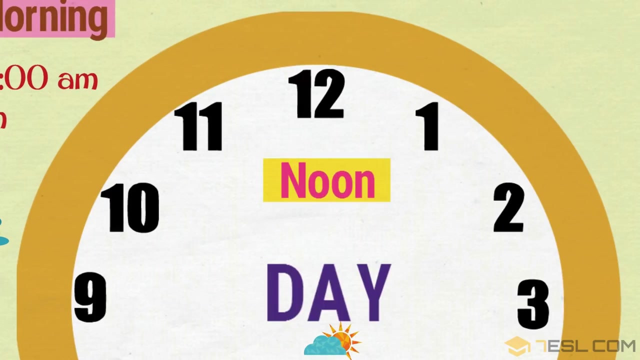 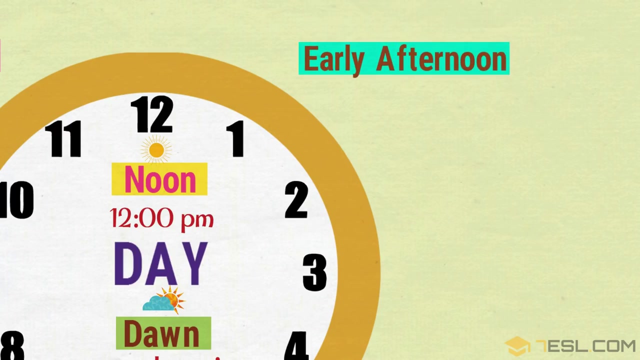 1.59.. MORNING: From sunrise to 12 o'clock pm. LATE MORNING: From about 10 am to 12 pm. NOON, EARLY AFTERNOON: From 12 pm to about 3 pm. 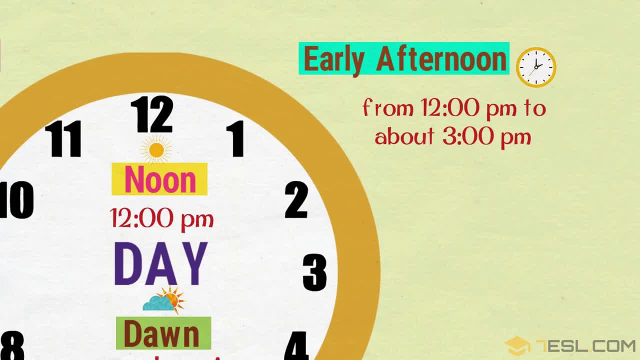 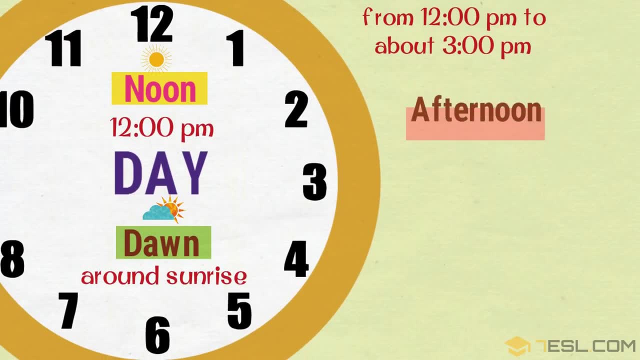 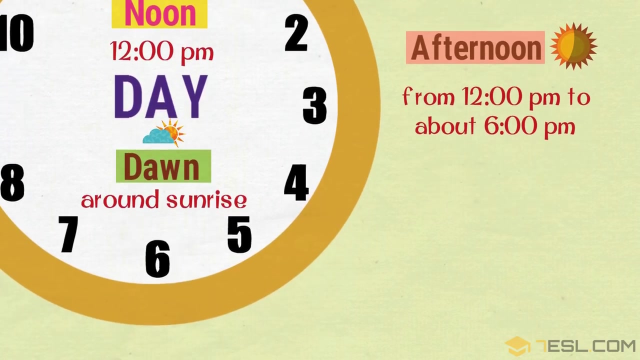 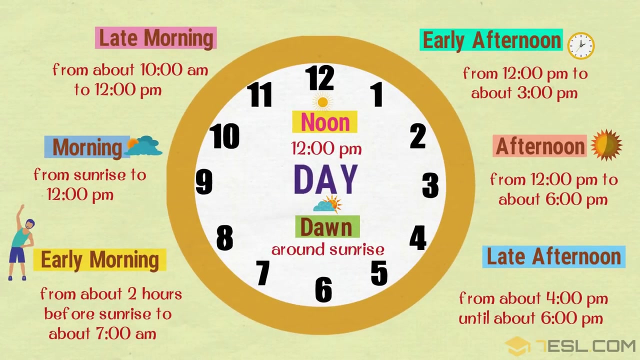 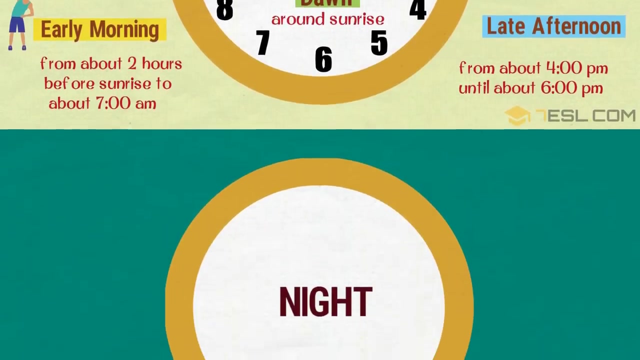 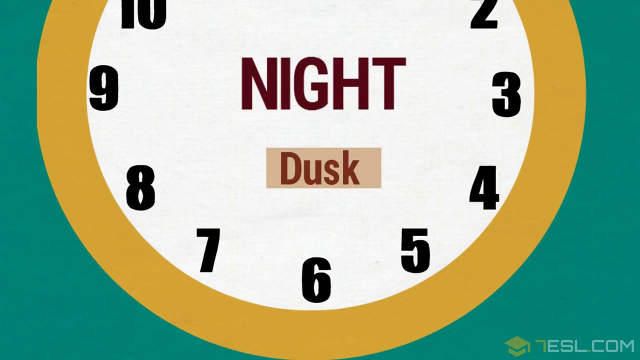 AFTERNOON From 12 pm to about 6 pm. LATE AFTERNOON. LATE AFTERNOON From about 4 pm to about 6 pm. AFTERNOON. NIGHT AFTERNOON- DUSK AFTERNOON.